We're also given the price of each. So let's say: this is the number and this is the price. Okay, So adult tickets cost $14 and children's tickets cost $11.. The only other information that we haven't used, that is that a total of $465 were paid for all these tickets. Okay, If we bought just one adult ticket, we would pay $14 for that. If we bought two adult tickets, we would pay 2x14, $28.. If we bought 10 adult tickets, that would be $14.. That would be $140. 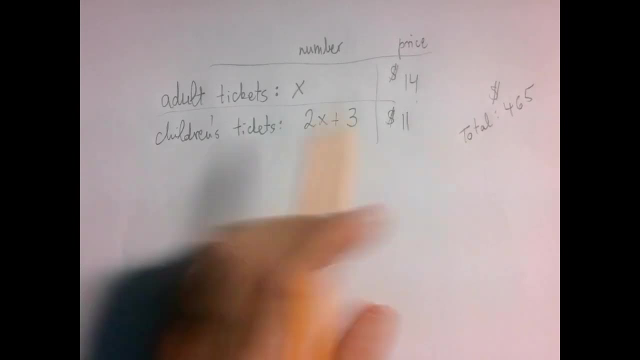 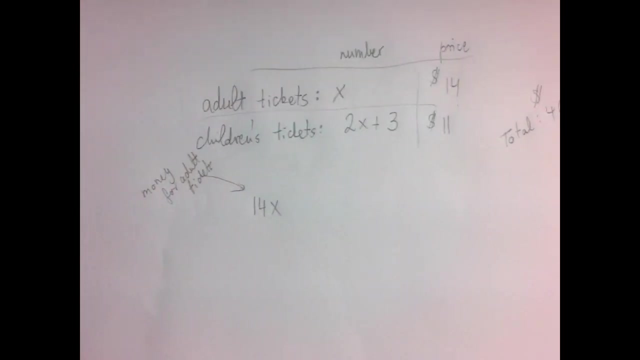 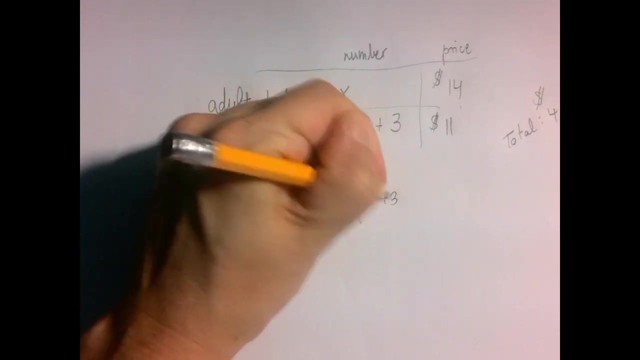 So x many adult tickets would cost 14x. So that's the money paid for adult tickets. Similarly, one children's ticket would cost us $11.. Two of them would cost $22.. Five of them $55. And 2x plus 3, many will cost us 11 times well, 2x plus 3 times 11.. 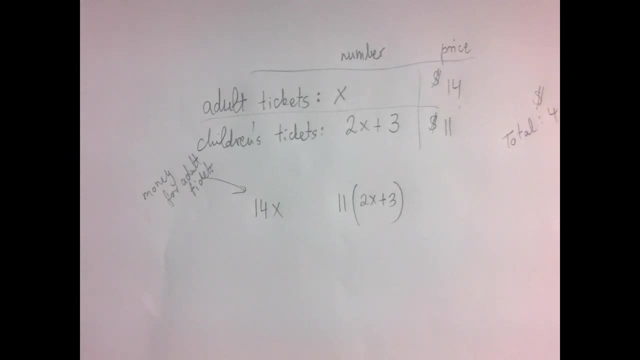 But our head is already at algebra So this is more familiar. So this would be the money spent on children's tickets, And if we add the two we would get the total price of all tickets, which is given to be $465.. 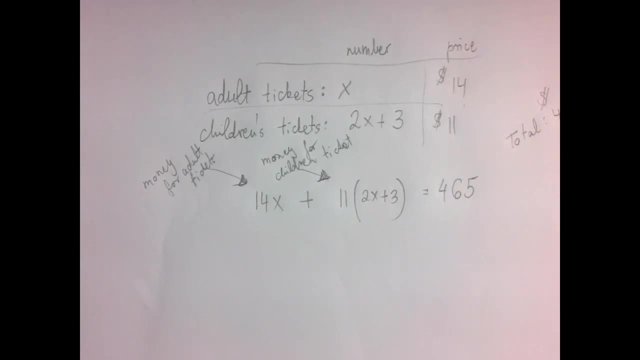 Now we have a linear equation in just one variable, so we can solve for x. Let's do that. We distribute 11.. We combine like terms And now it's just a two-step equation. We're going to subtract 33 and divide by 36.. 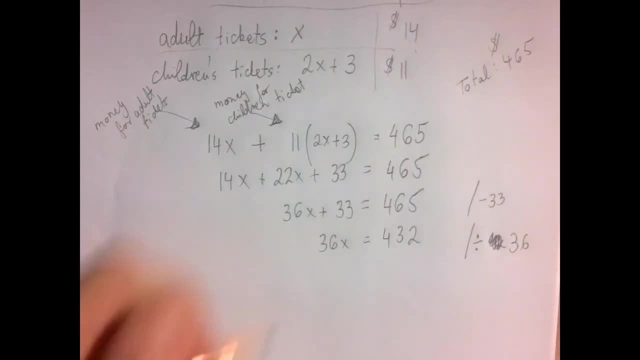 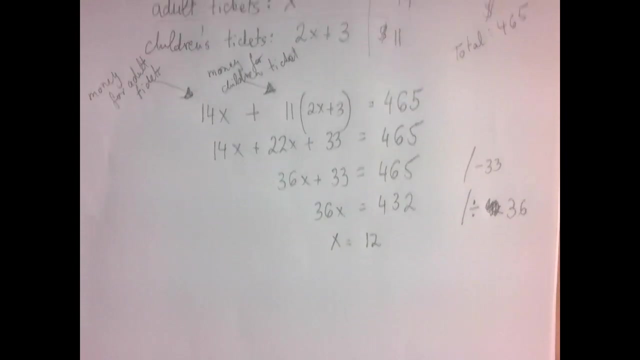 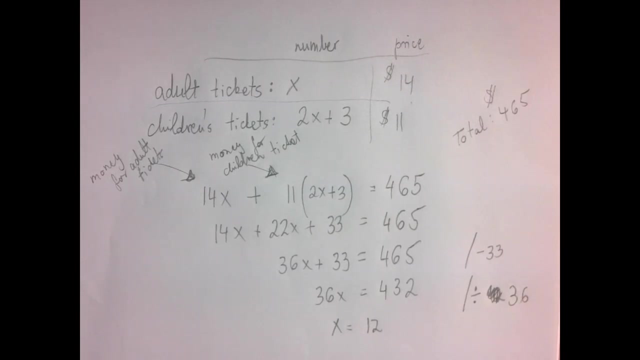 So x is 12.. Which would be the end of the problem if we were asked about x given an equation, But we were the ones setting up the equation. We are in the middle of a word problem, So we should probably read what they ask us to return. 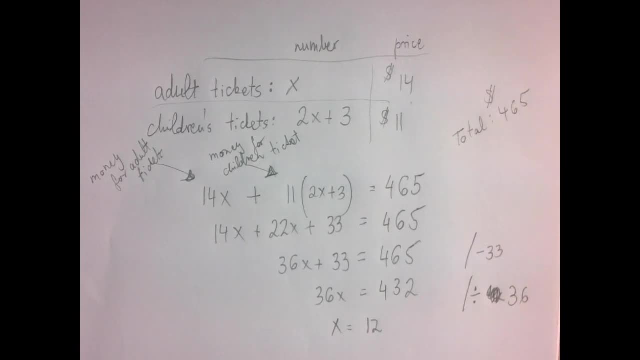 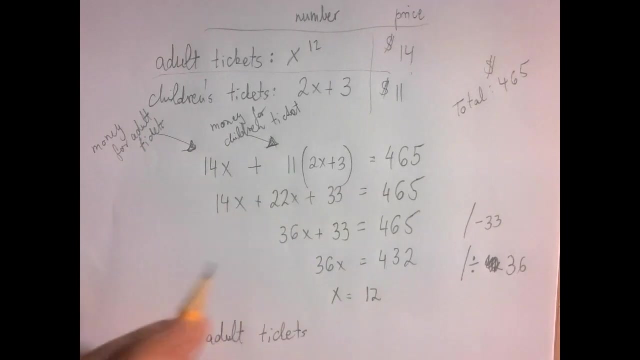 The question is how many children's tickets and how many adult tickets were bought. Well, if x is 12,, that means that we have 12 adult tickets, And the number of children's tickets is an expression also in x. That x is also 12.. 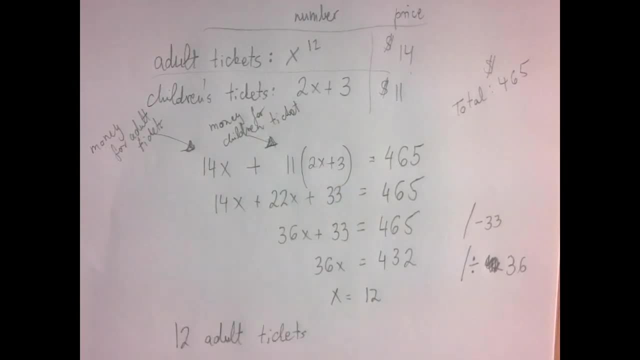 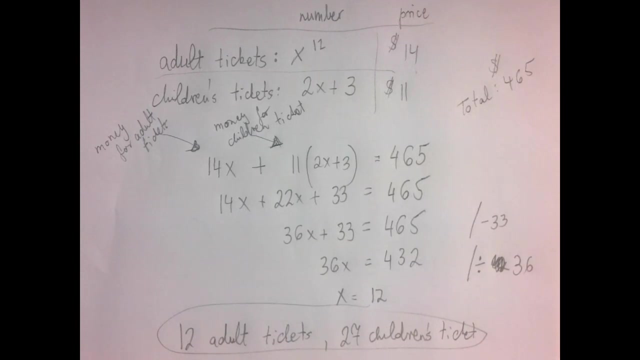 So we're talking about 2 times 12 plus 3.. That's 27 children's tickets. Once we have the answer, let's check. So how much money would we pay for the adult tickets? It's 12 of them and each of them costs $14.. 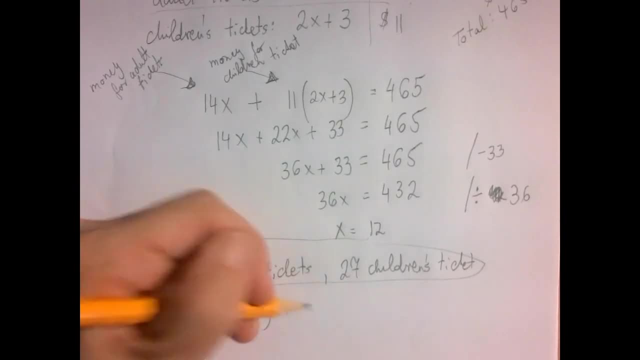 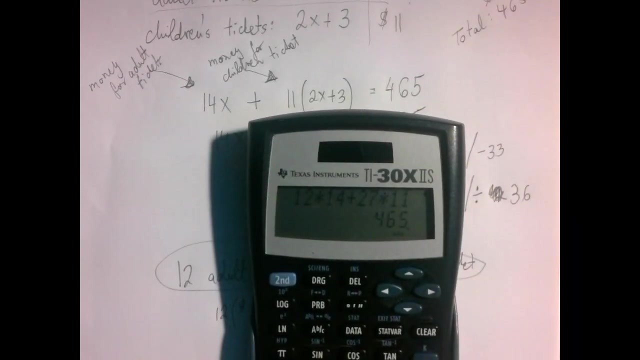 And for the children's tickets we would buy 27 tickets, each of them costing $11.. So if these two add up to $465, then we're in good shape. There it is, But the only other thing we could check for is the comparison.